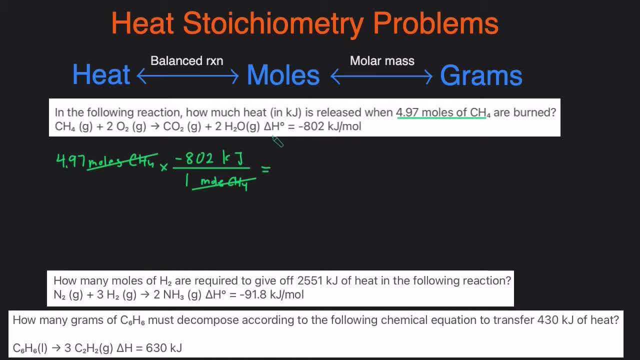 So we just plug this in the calculator: 4.97 times negative 802, and then that will give us negative 3,900. And 90 kilojoules if we take it to three sig figs. So that's how much heat we'll be giving off, and this negative just means that energy is released. 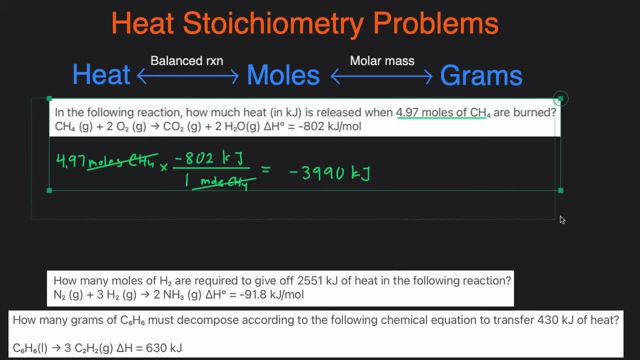 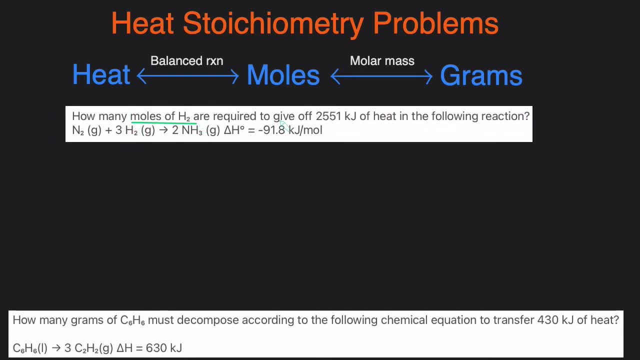 That's the first example. let's take a look at the next one. So in the next one we're asked to solve for the moles of H2 that are required to give off 2,551 kilojoules of heat in this reaction. 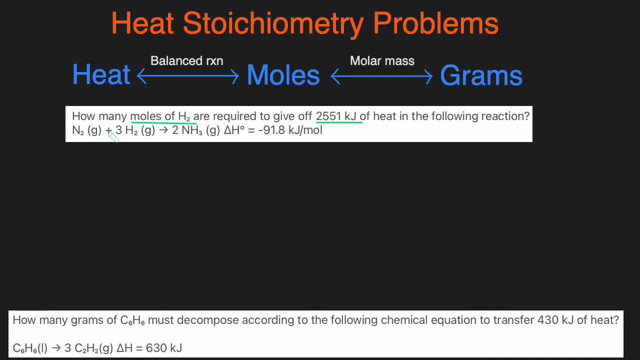 So once again we have a reaction. You have to just make sure it's balanced. So we have a reaction with a delta H that's given and then we're asked to solve for moles. So that's an indication. this is a heat stoichiometry problem. 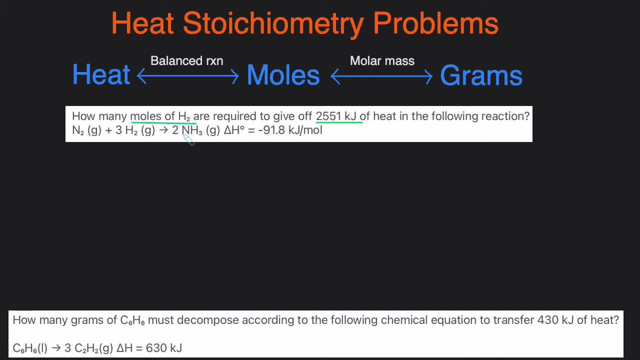 We start off with the number that's given. that's not part of the chemical reaction, So not the delta H, but the heat that's given off. So we'll put 2,551 kilojoules. That's what we started with. 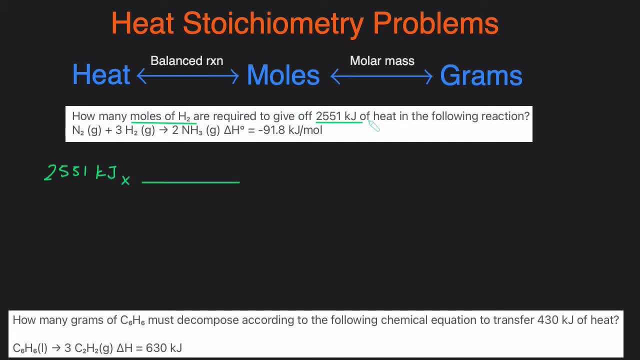 Multiply it by the conversion factor. So this time we have heat and we want to get to moles. So it's just a mole, It's a one-step conversion And we'll put kilojoules on the bottom. So whatever you started with goes on the bottom, so it can cancel out. 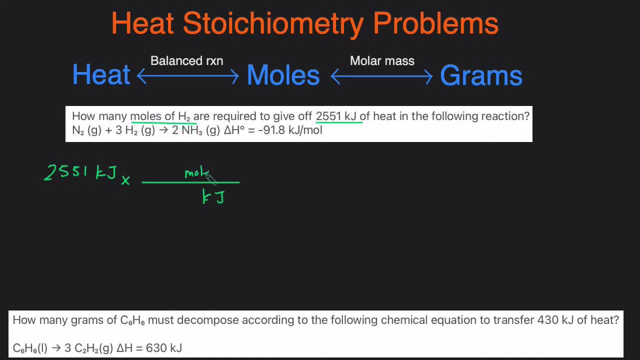 And we want moles of H2, and that's what's going to go on the top. Then we take a look at the chemical reaction. How many moles of H2 do we have in this reaction? We have 3 moles of H2.. 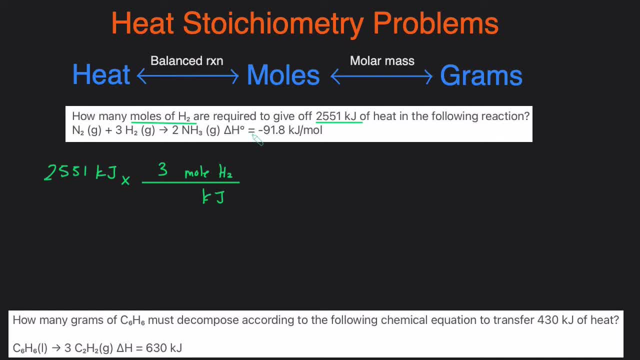 So we'll put 3 moles on top. And how much heat do we have in this reaction? We had 91.8.. I'm dropping negative. So in the end you can't have a negative amount of moles. That's why I dropped the negative. 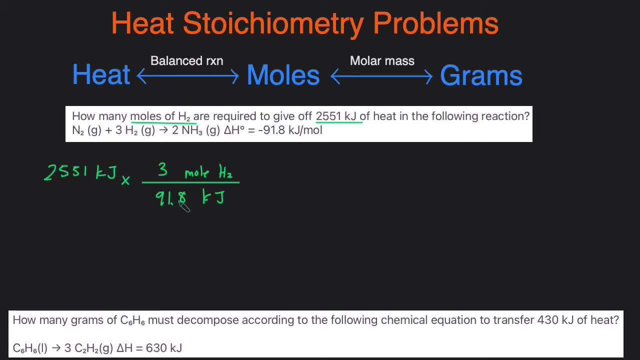 Because if we kept the negative here, then our answer is going to be negative. So you just want to make sure that the grams and the moles is always positive in the end And then, when we do that, you can see that the kilojoules cancel out. 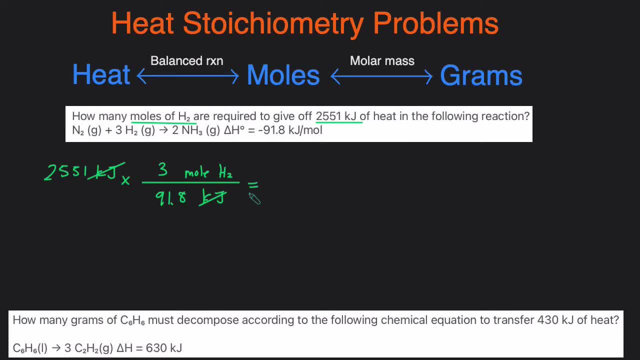 And we can just enter this in the calculator: 2,551 multiplied by 3, divided by 91.8.. And then our final answer would be 83.337.. Because of four sig figs: Moles of H2.. And that's the answer for the second question. 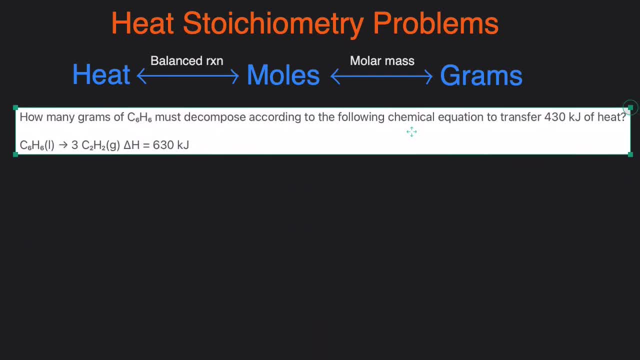 Let's take a look at the last question. So in this last question we're asked to solve for grams of C6H6,, which is benzene that must be decomposed to transfer 430 kilojoules of heat, And then we have a reaction with the delta H. 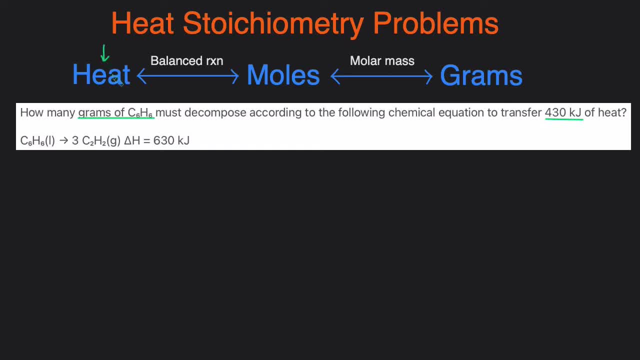 So this time we are starting here. We're starting at the heat And then we're moving all the way to the grams. So this is going to be a two-step conversion. Previously we've only seen one-step conversion to the heat and moles. 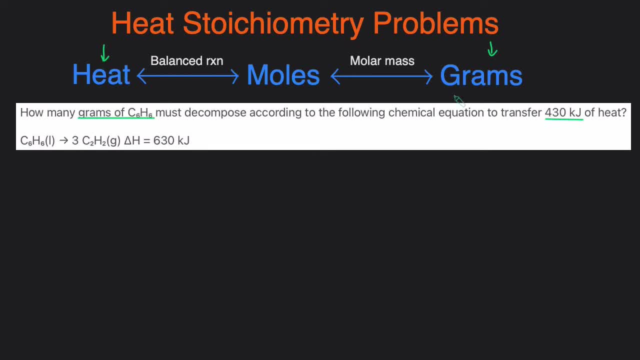 Now we're starting from heat And then we're going all the way to grams. So we'll start with the given, which is 430 kilojoules of heat, And then the first step that we have to do is we have to convert the heat to the moles. 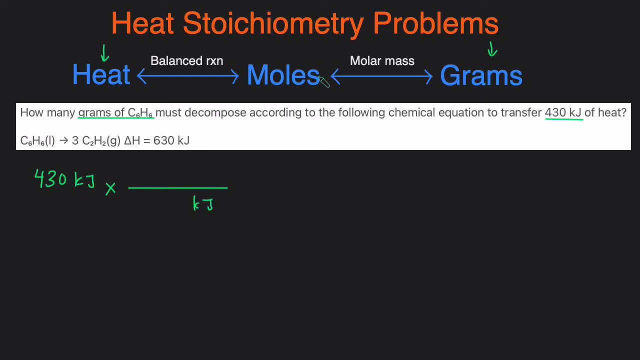 So we got to get rid of the heat. So we put the kilojoules on the bottom And then we want to get the moles, specifically moles of C6H6.. So we'll put moles of C6H6 on the top. 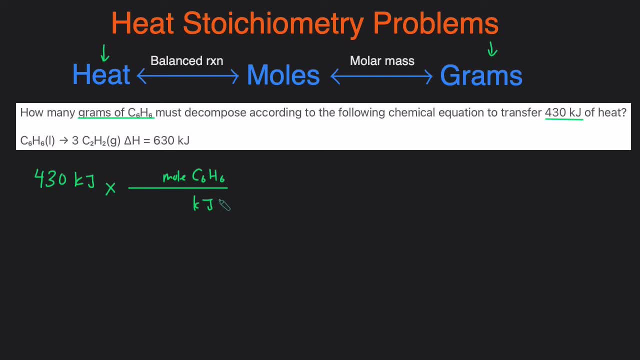 Because whatever you're trying to go to goes on top, Whatever you're trying to get rid of goes on the bottom. And we look at the balanced chemical reaction And in this reaction we see there's one C6H6.. So we put that here. 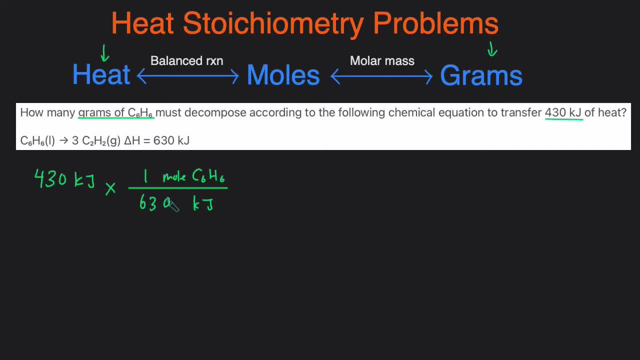 And then how many kilojoules is in the reaction? 630.. After the first step, the kilojoules disappears And then now we have moles of C6H6. And then you want to get the moles. 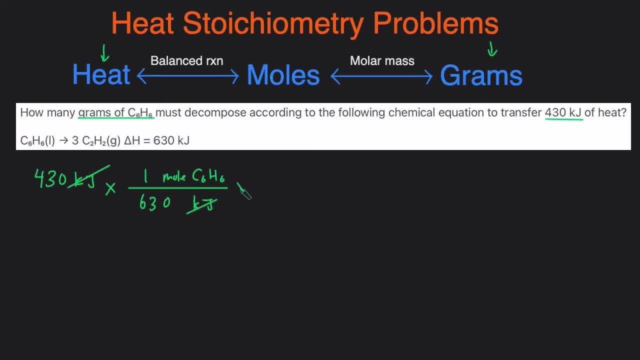 And then we want to get the moles, want to convert to grams. so this is the second conversion. then we multiply by another conversion factor, put moles of the benzene on the bottom, so then that way it can cancel out. and we're trying to get the grams. so we'll put grams of c6h6 on the top and then, for this part, we just